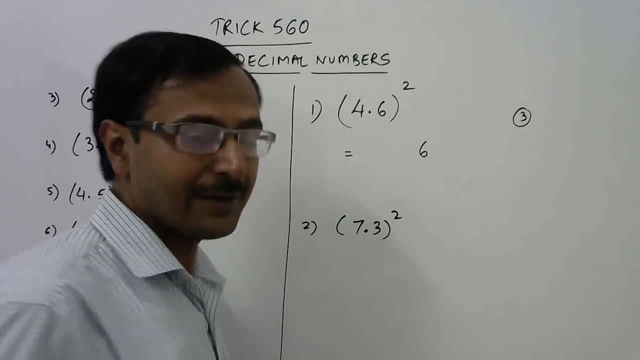 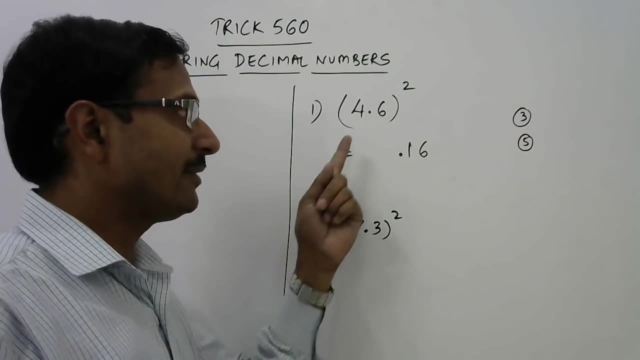 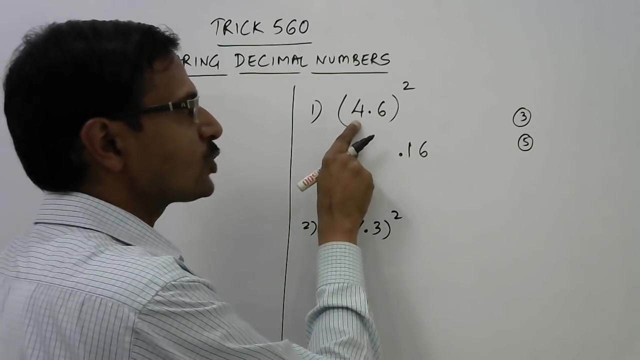 Double that product, So 24, and the double is 48 and plus 351.. 5.6 square is on the né mobile, 5.5 square is on the choose. then you have 2 digits, any bar just below the bar, But all double that little of it change. Total square is 15.. But 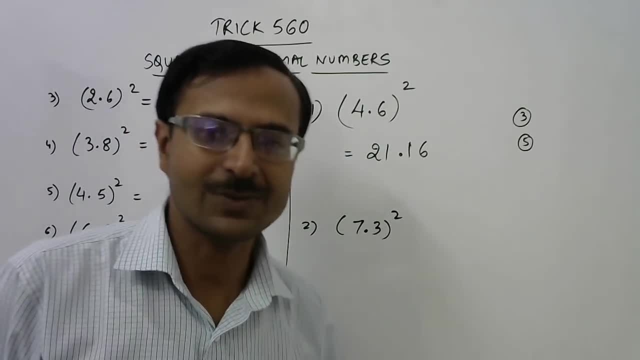 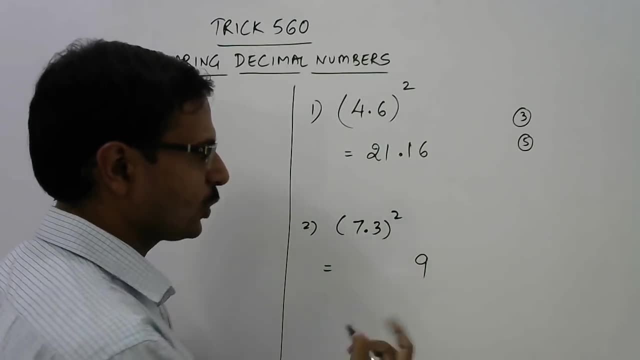 21.. So here you have the answer: 21.16 is the square of 4.6.. Let us demonstrate this method once more Now see: 3: square is 9.. So no carries 7, 3 is a 21.. Double is 42.. So 2 and 4 carry. 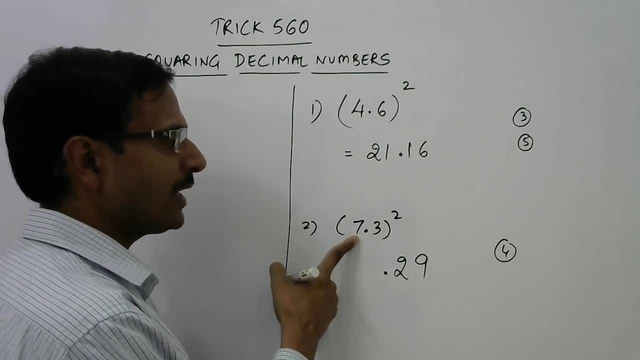 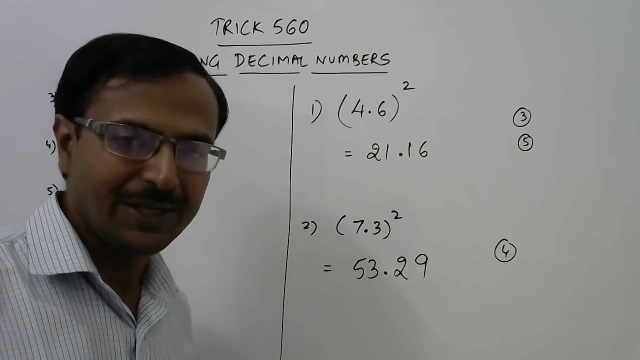 Now you put the decimal and finally, 7 square is 49.. 49 plus 4 is 53. So 53.29 is the square of 7.3.. I hope you have understood this method and, if you have understood this, now solving all these. 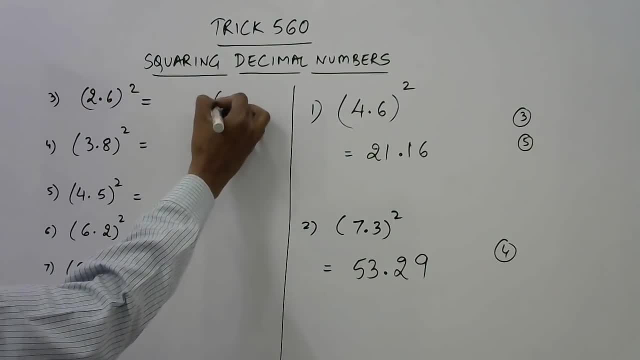 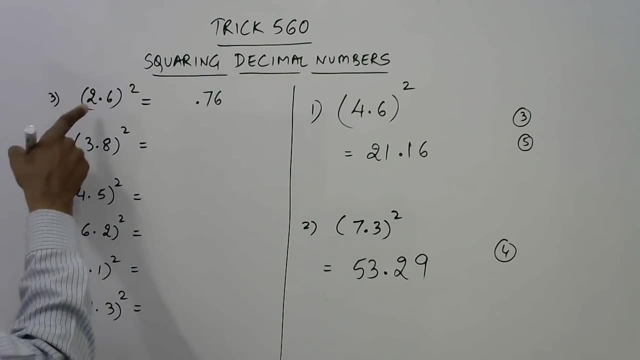 problems will be very easy. Let us see: 6 square is 36.. So 3 carry 6 to the 12,, 24 plus 3, 27.. 2 carry 2 square is 4 plus 2, 6.. 8 square is 64.. 4, 6 carry 24, 48 plus 6, 54.. 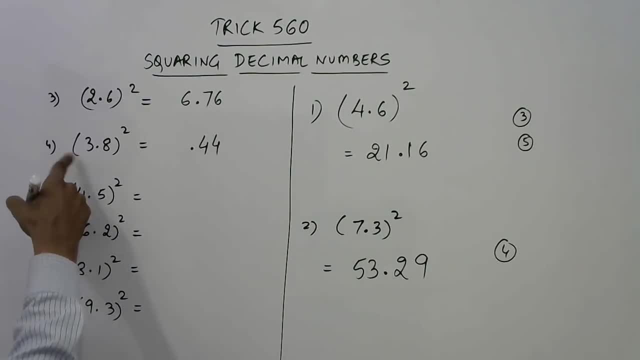 5 carry 3 square is 9. 9 plus 5, 40.. 5 square 25.. 5, 2 carry 20, 40,, 42.. 4 carry 4 square 16 plus. 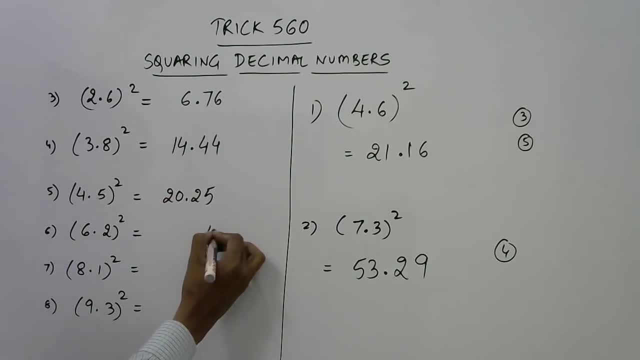 4, 20.. 2 square is 4.. 6 to the 12, double is 24.. 2 carry 6, 6 are 36.. 38.. 1 square is 1.. 8 into 1,. 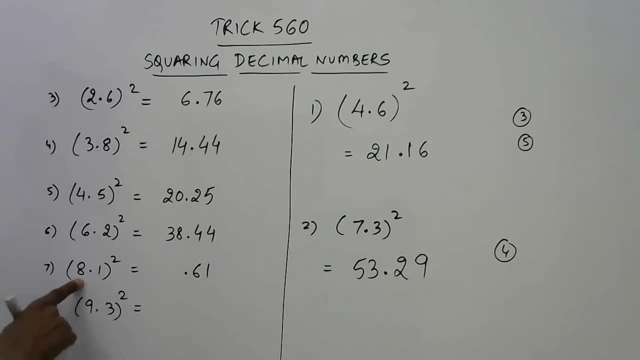 8. Double is 16.. 6.. 1 carry 64 plus 1, 65.. 3 square is 9.. 9, 3 is a 27,. 54.. 5 carry 81, 86.. So 86.49.